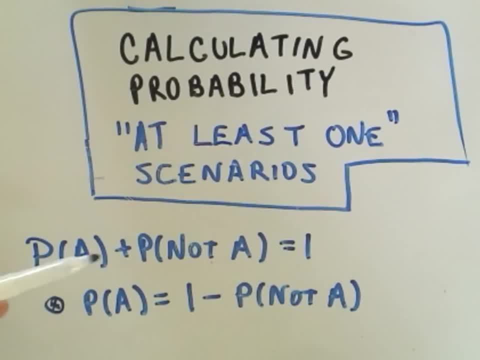 you know the probability of some event A happening plus the probability of it not happening. well, either it does or it doesn't. so the probability of something happening plus the probability of it not happening has to add up to 1 or 100%. 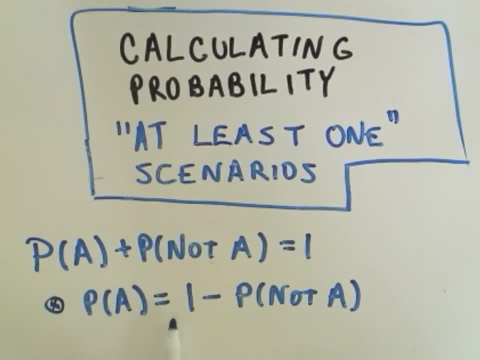 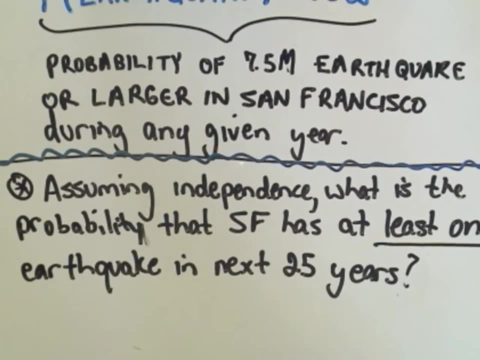 So basically it says the probability of A is equivalent to 1 minus the probability of not A, and we're going to use this formula in the next part. So I was digging around on the good old Internet and I don't know how truthful this data is. 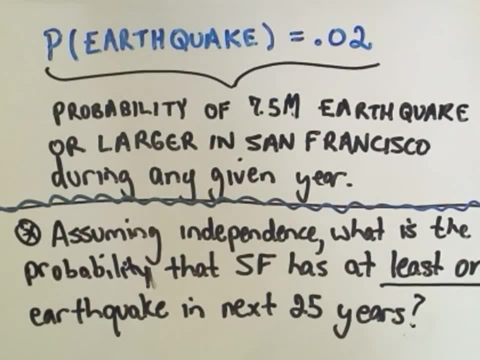 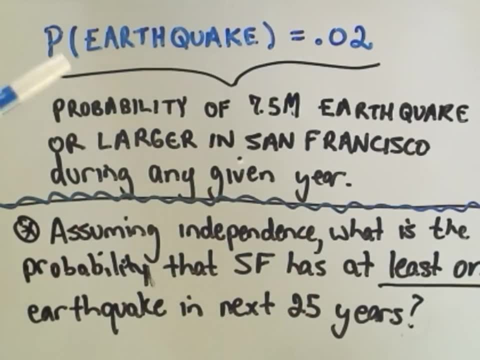 but I saw it in quite a few places. It looked reliable on the sites I saw it. So it says the probability of an earthquake, a major earthquake, a 7.5 magnitude or greater, during any single year in San Francisco. it says the probability of that is 0.02 or 2%. 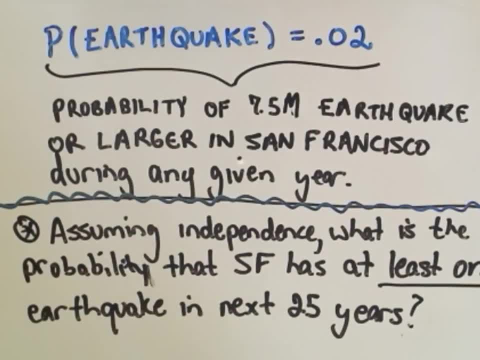 So you know 2%. you know it always depends on the situation whether it sounds like a lot or not. you know not very much. If the odds of me winning a game were 2%, I wouldn't think, you know, that was very great. 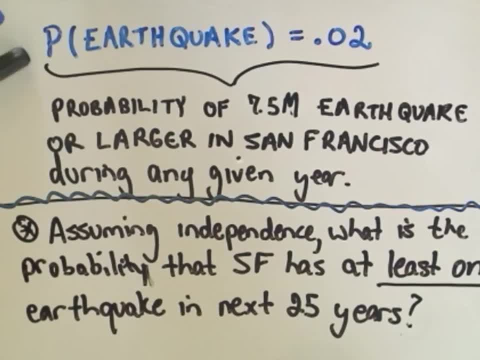 But you know, if you're living in San Francisco, the probability of an earthquake being 2%. if I was the mayor, I would be very, very concerned with that. That sounds like a pretty high percentage to me because if it does happen, bad things are going to happen. 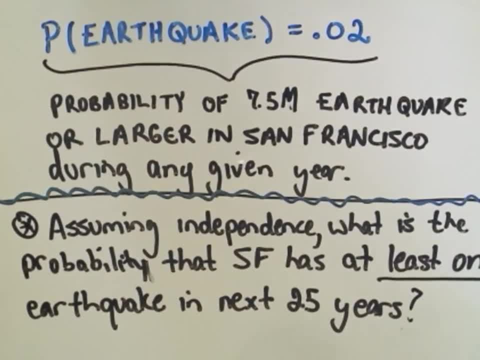 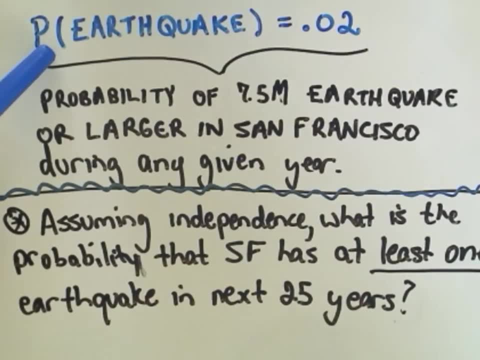 And if you've ever been to San Francisco, you know that they take this very seriously. So what we're going to do here is based on this data, and I doubt this would probably be the case, but let's assume, just to make our mathematics work out here. 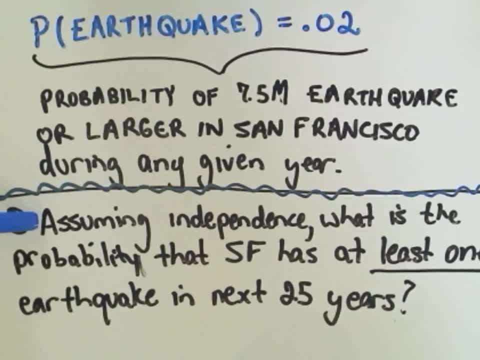 that whether an earthquake happens from one year to the next in San Francisco are independent events, And I find that very hard to believe that they would be independent events. But again, just for the sake of our computations, let's assume they are independent events, okay. 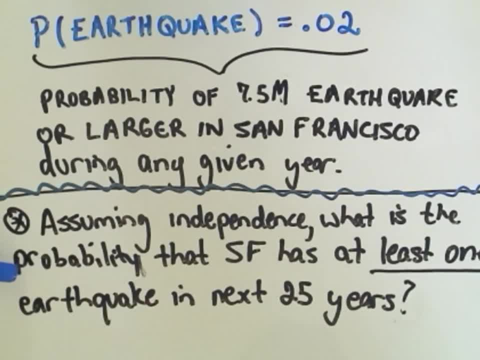 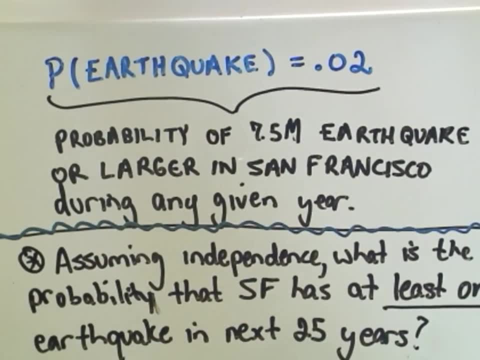 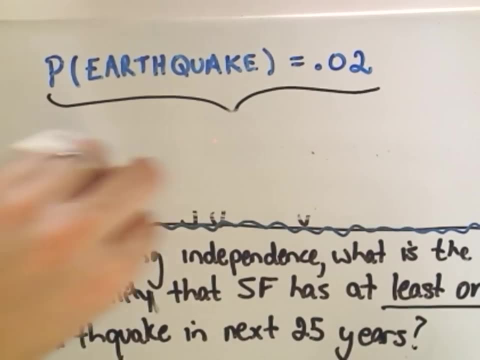 So, assuming that we want to calculate the probability that San Francisco has at least one earthquake in the next 25 years, Okay, so we went under the probability It has at least one 7.5 magnitude earthquake. Okay, well, the way that we're going to do this, 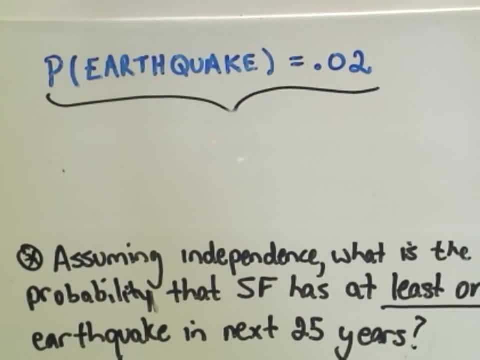 you could calculate it directly, and you could calculate the probability that San Francisco has exactly one major earthquake, plus the probability that it has exactly two, all the way up to the maximum number, which would be 25.. But instead, we're going to think about this as being our event A. 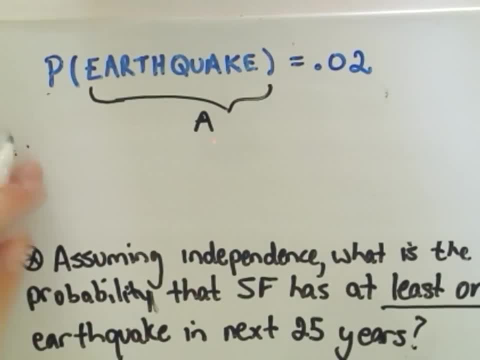 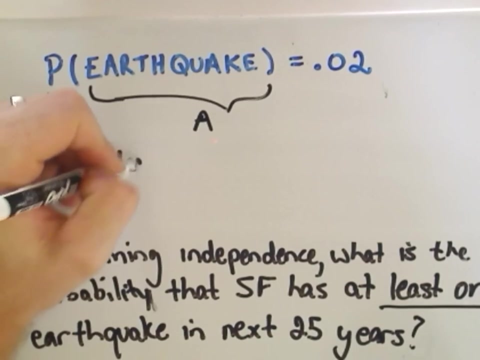 Okay, so A is going to be the event of having an earthquake. Well, we're going to calculate that by using 1 minus the probability. So okay, excuse me, I'm getting ahead of myself. So, first off, we're trying to calculate the probability of at least one earthquake. 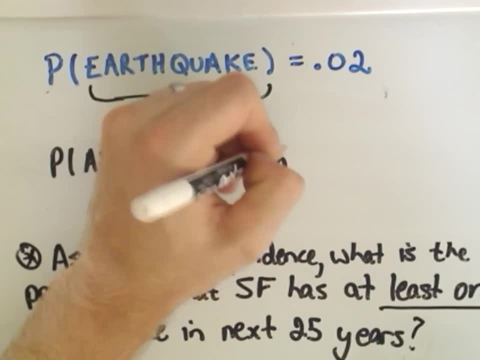 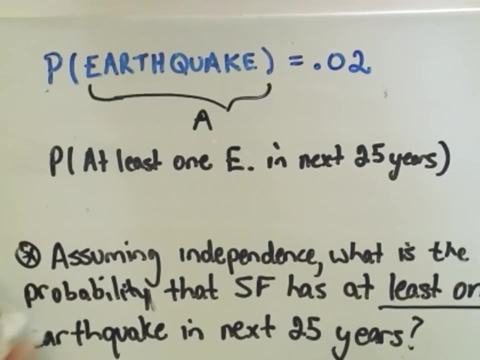 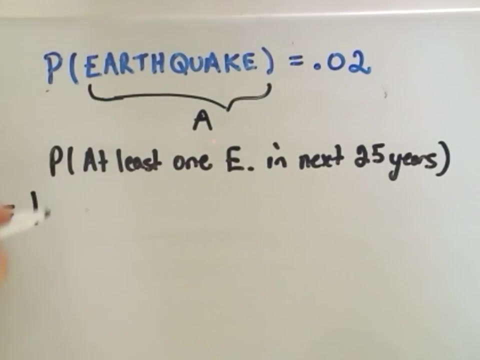 At least one earthquake in the next 25 years. So I'm going to abbreviate some stuff here as I go, because these can get wordy. Okay, At least one earthquake in the next 25 years. Well, here's where I'm going to use my 1 minus P of, not A. 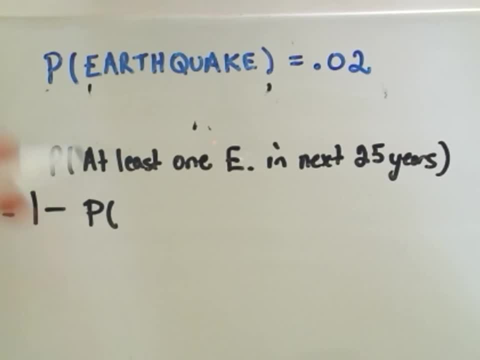 So let's think about this event A. Our event A is going to be having at least one earthquake in the next 25 years. Well, the negation of that. if that doesn't happen, if there's not at least one earthquake, that means there are no earthquakes. 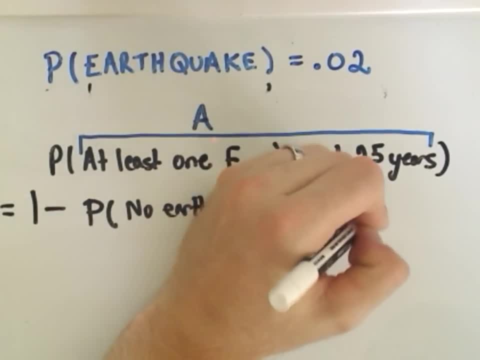 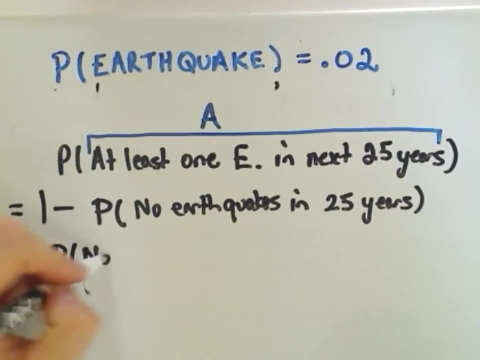 In the next 25 years. Okay, and really this is an and statement, because what happens if there's no earthquakes in 25 years? It says really what's going on. there's no earthquake, So there's no earthquake in the first year. 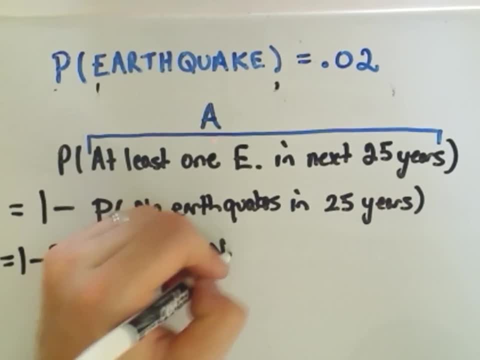 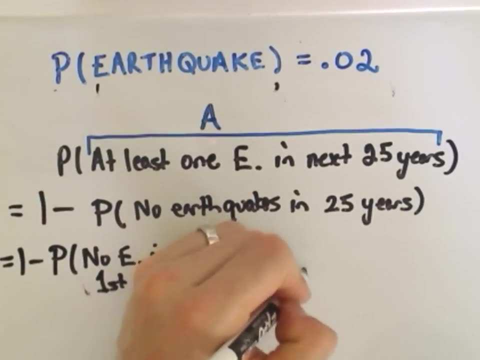 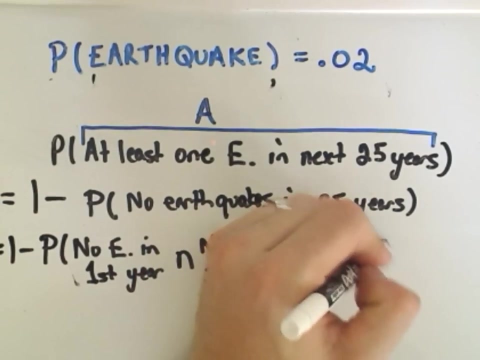 And there's no earthquake in the second year, And there's no earthquake in the third year, fourth year, fifth year, all the way up to Eventually, there would be no earthquake in the 25th year. Right, That's really what it means if there's no earthquakes in 25 years. 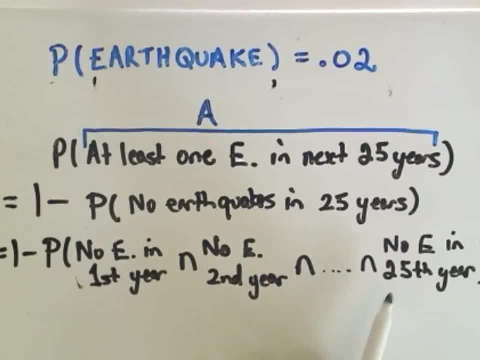 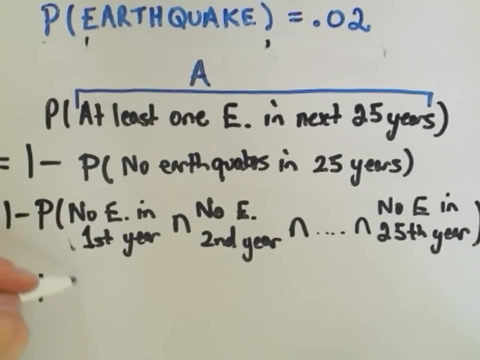 There wasn't one in the first year and the second year and the third year up to the 25th year. Well, now we can calculate this probability directly, because it says this is going to be 1 minus The probability there's no earthquake in the first year. 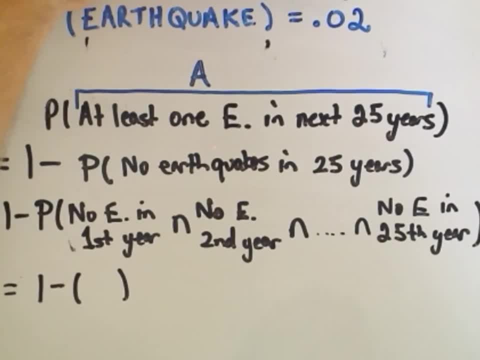 Well, we said that during any given year, there's a 0.02 probability of there being an earthquake. Well, that means during any given year, there's a 0.98 probability that there is no earthquake. Likewise, the probability that there's no earthquake in the second year would be 0.98 times 0.98.. 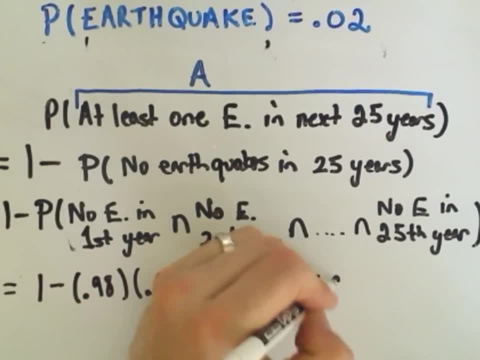 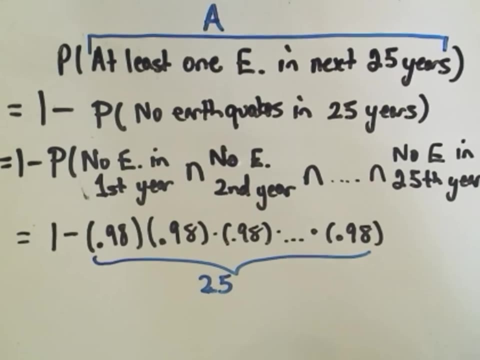 We would do this a whole bunch of times- 0.98. This would be in year 25.. Okay, so what do we have? We have 25.98 being multiplied together. So it says the probability of us having at least one earthquake in San Francisco in the next 25 years. 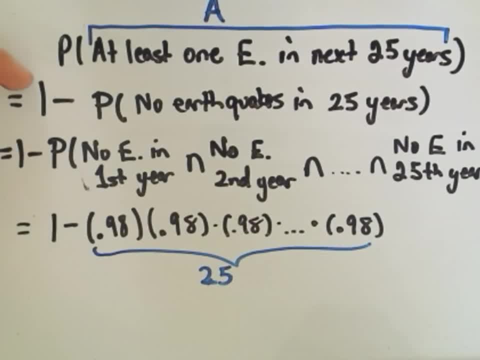 is the same thing as finding the probability of calculating 1 minus the probability that there's no earthquakes in 25 years. It says that's equal to 1 minus 0.98.. 0.98 to the 25th power, which I calculated to be roughly 0.397. 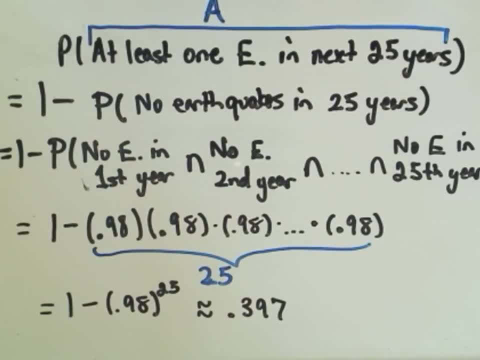 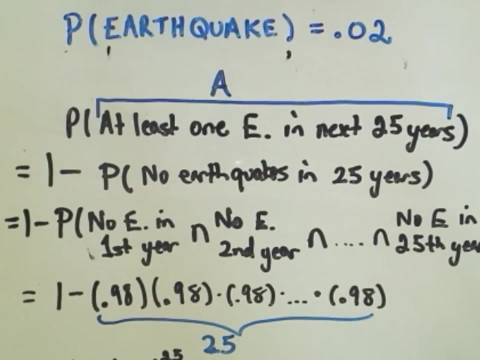 So there's about a 40% probability that there'll be at least one 7.5 magnitude quake or higher in the next 25 years. based on my probability that in any given year the earthquake happening is 2% And again also assuming independence. 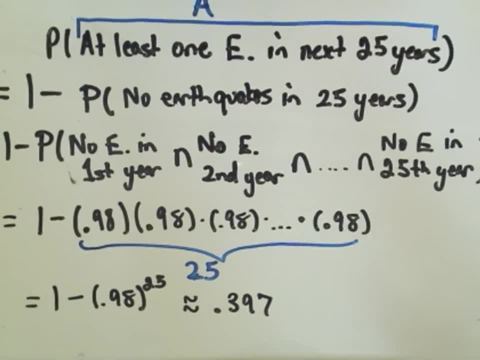 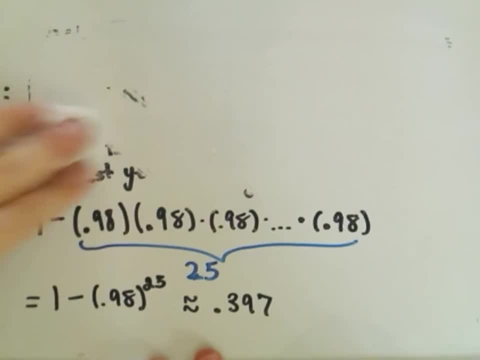 That's a big, important notion. okay in this one. So you know, next 25 years, hey, if you settle down there and you plan on living there, 40% you know. that to me is pretty significant. 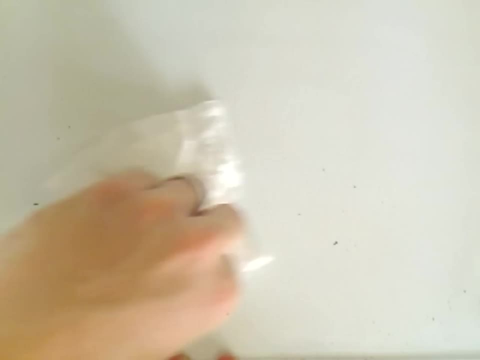 You know I would again. that's something I would take very seriously. Likewise, just for my own sake, I don't know. I thought maybe it was interesting if you calculate the probability of at least one earthquake in the next 50 years in San Francisco.